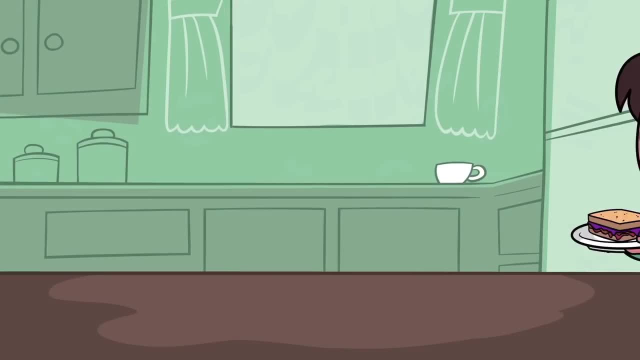 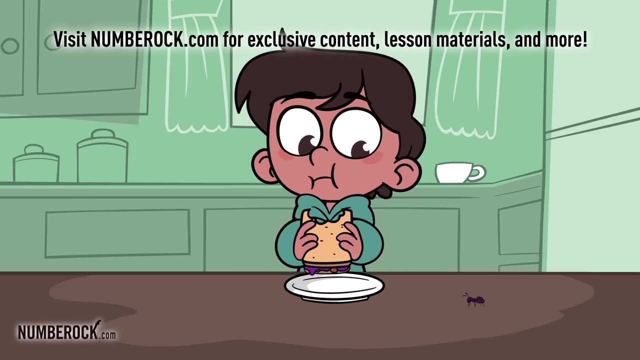 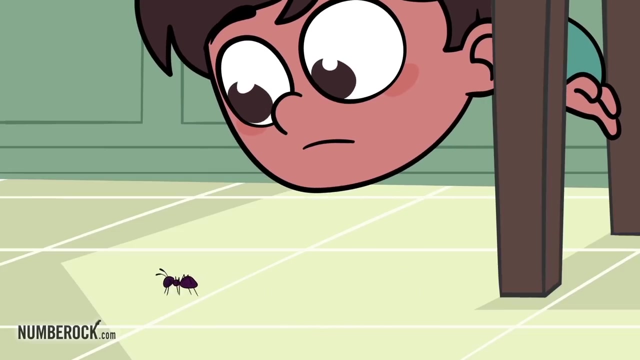 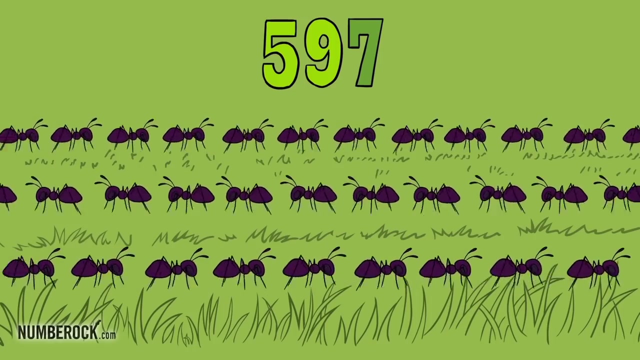 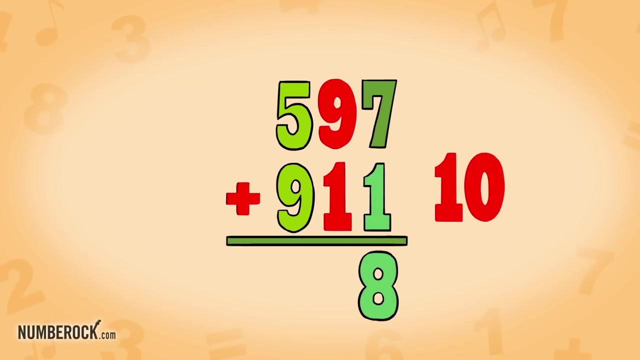 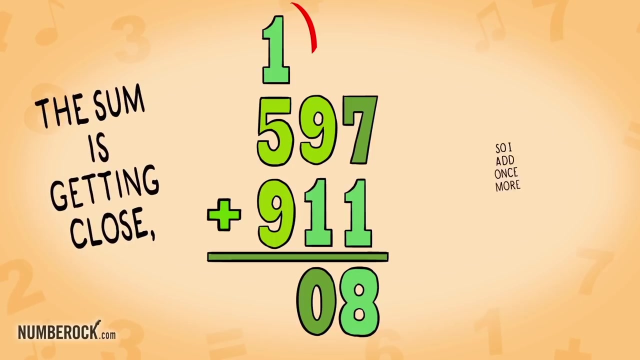 597 ants above ground Plus 911 ants underground. 7 plus 1 is 8, 9 plus 1 is 10. Each one of them is my special insect friend. Zero stays on the floor. the hundred heads next door. The summer's getting close, so I add once more: 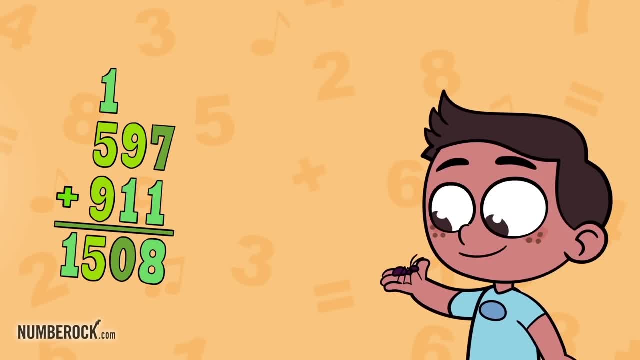 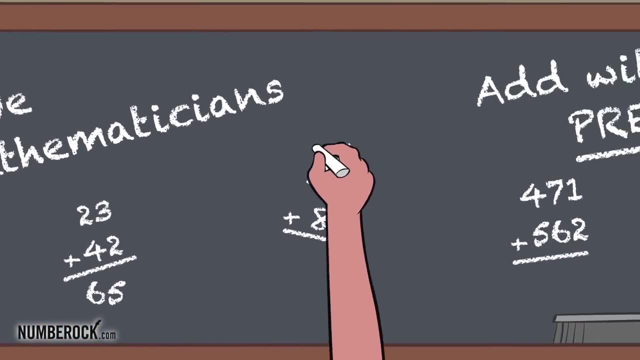 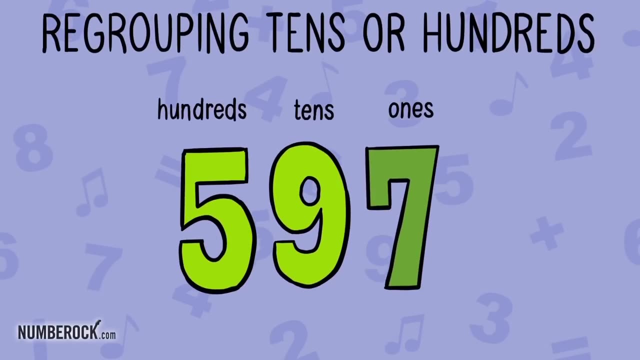 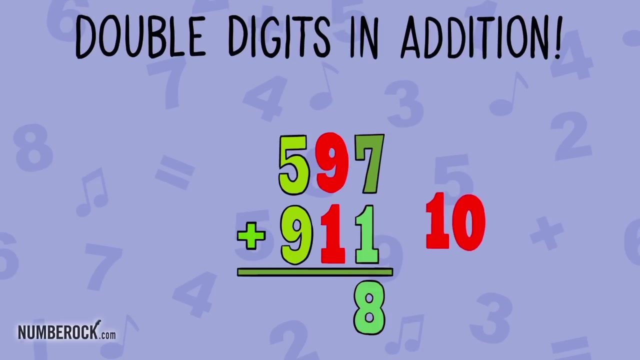 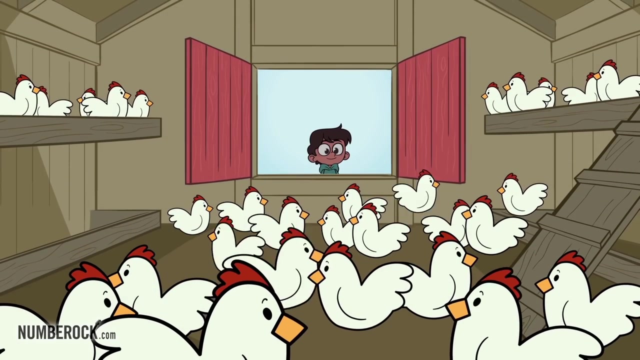 1 plus 5 is 6 Plus 9 is 15. My little brother thinks they're a good source of protein. We mathematicians Add with precision, Regrouping, Tens or hundreds when We find double digits. in addition, 189 hens are inside. 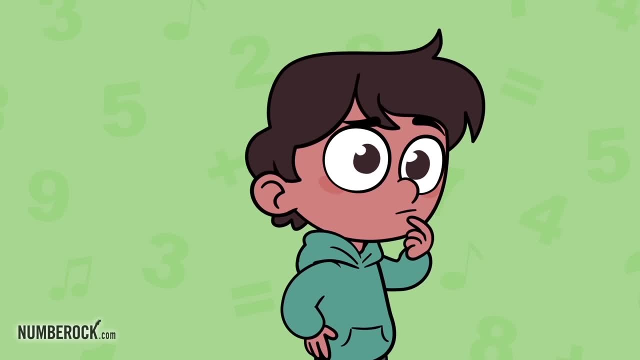 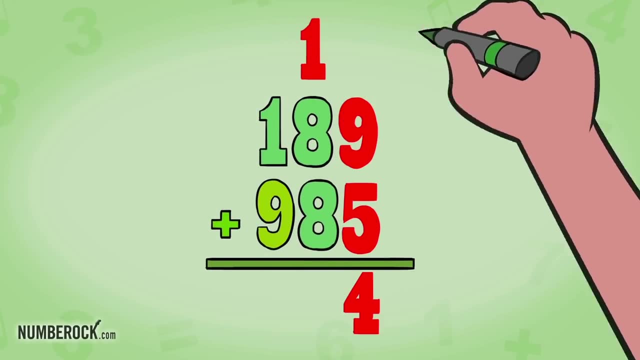 And 985 hens are outside. To find out how many hens are in the coop, We gotta know how to add and regroup 9 and 5's 14, right for the 10 carries. 1 plus 8 is 9, plus 8 is 17. 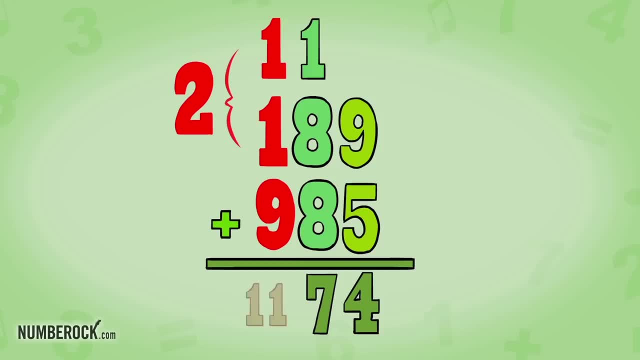 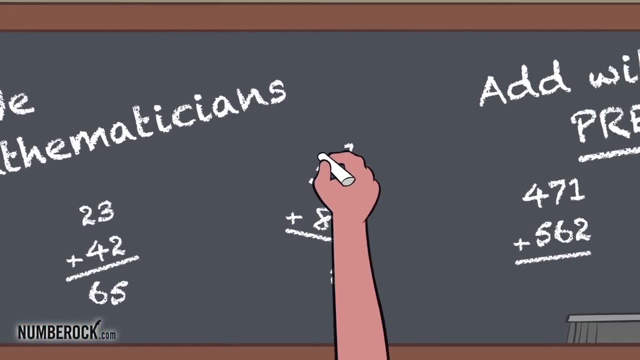 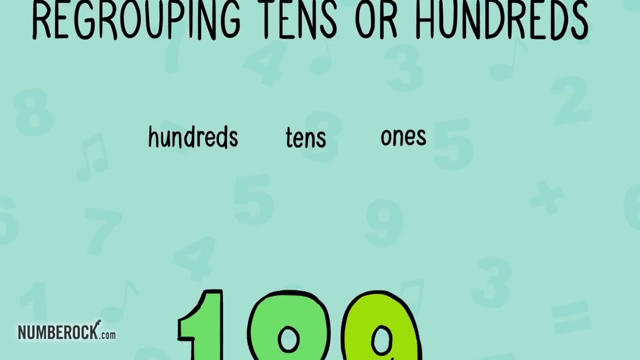 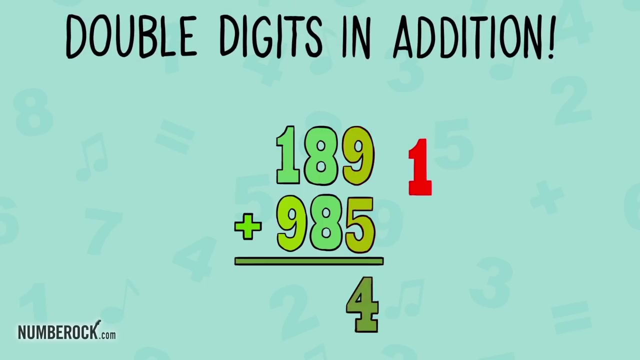 Keep the 7, the hundred regroups 2 plus 9 is 11, cock-a-doodle-doo. We mathematicians Add with precision Regrouping tens or hundreds when We find double digits. in addition, Sometimes we make errors. it's inevitable. 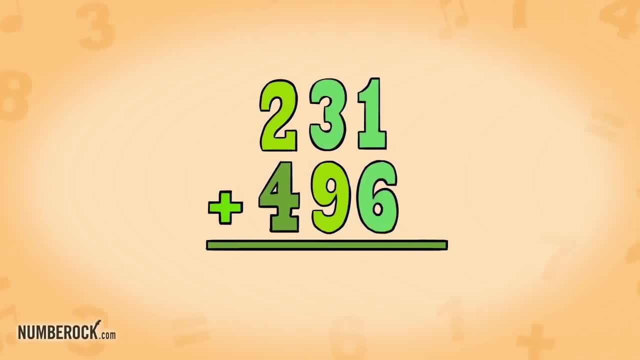 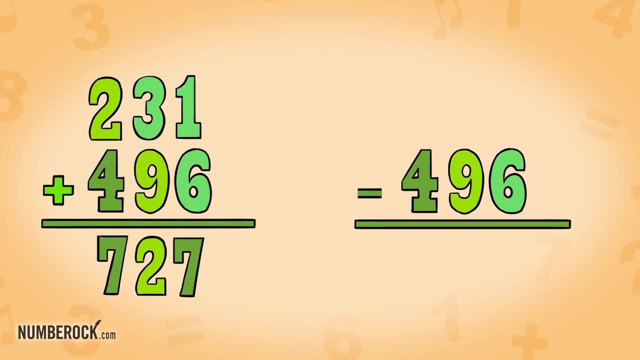 But check your work and it'll be in time, It'll be intuitable. The best way to check your addition Is by subtraction, the inverse operation. Take either addend and subtract from the sum. If you get the other addend, your work is done.